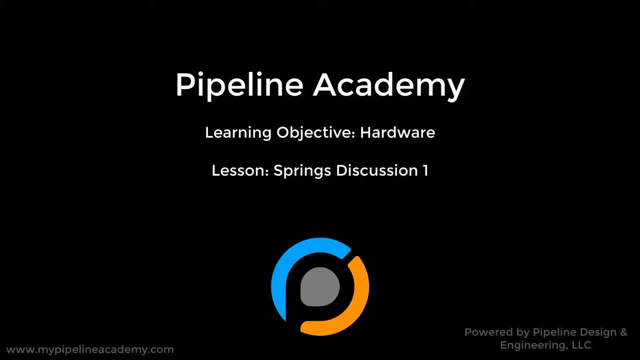 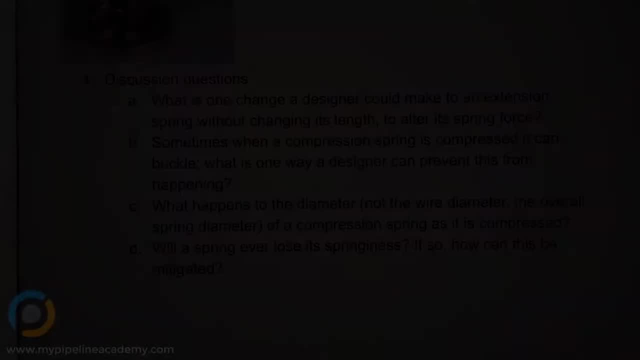 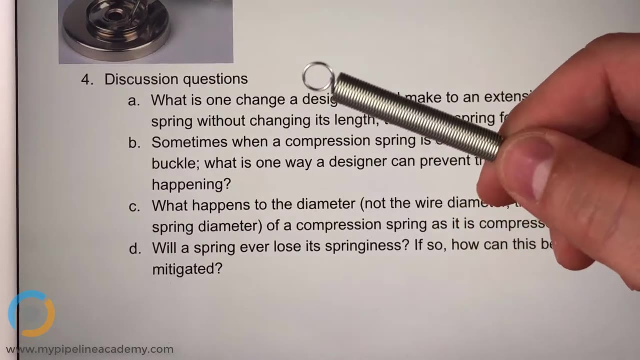 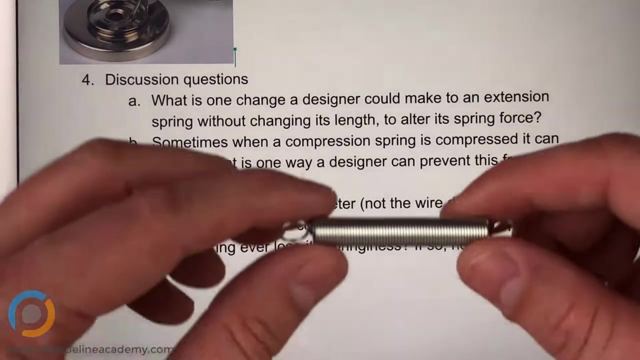 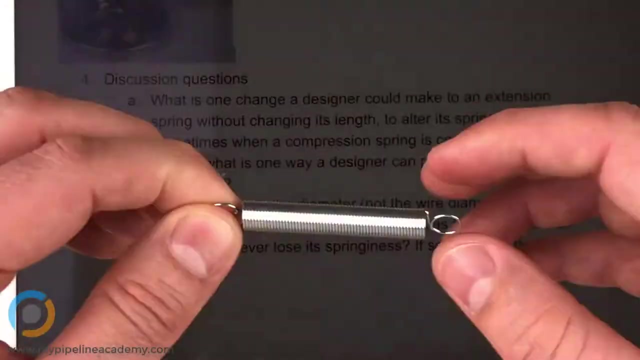 What's one change a designer could make to an extension spring without changing its length to alter its spring force? or maybe a better way of saying it is to alter its spring constant. So what's one change we could make to the spring without changing its length that would? 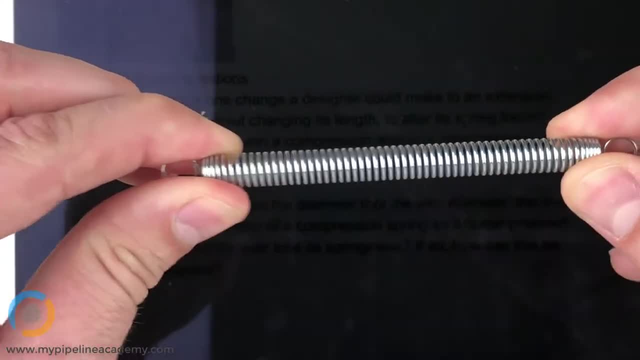 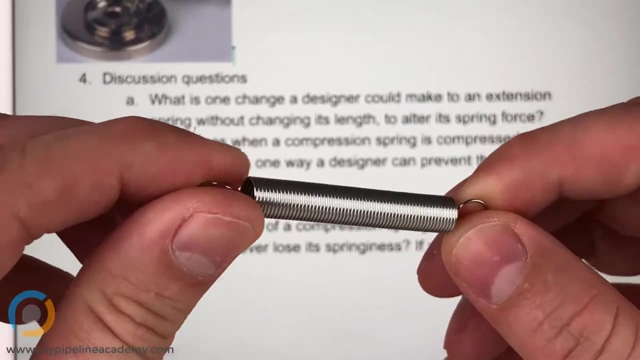 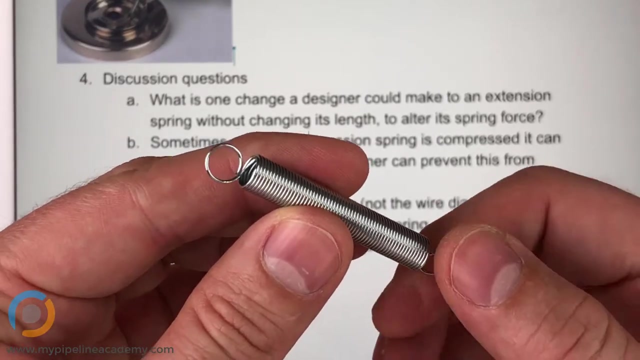 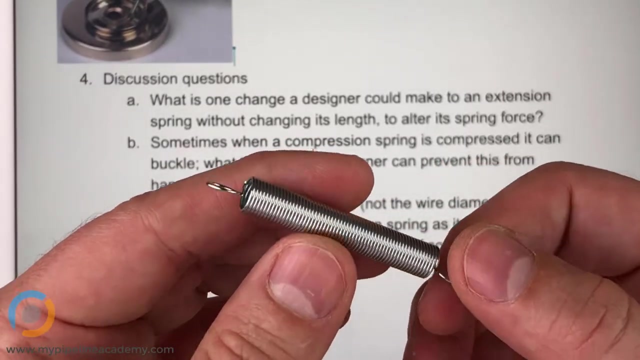 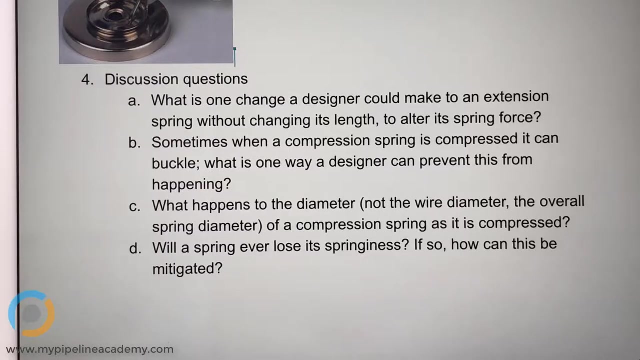 change the amount of force that is realized when you pull it apart. I have no idea. Think about the diameter of the wire used. I was thinking: get a new spring altogether. That's what's going through my mind. So I've got a pair of calipers here. 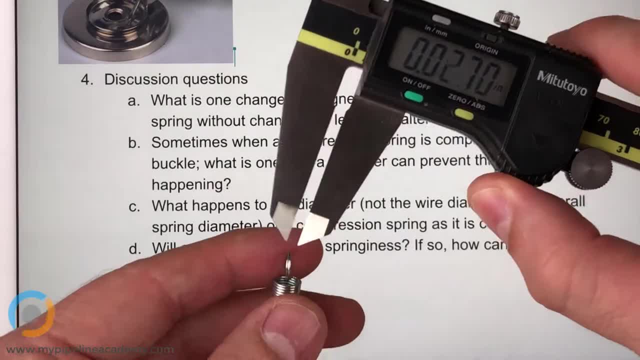 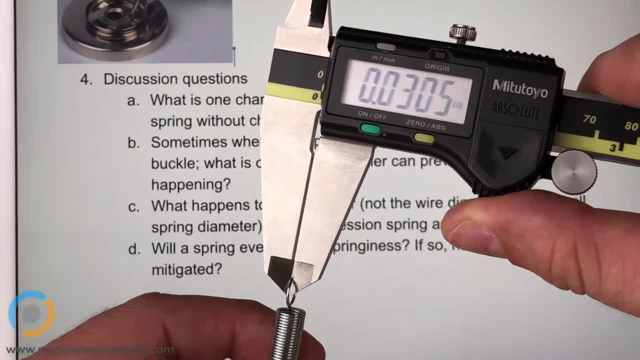 This is just a tool used to measure distance or thickness. And if we measure the thickness of that wire we see it is about 30 thousandths of an inch. So one thing we could do to increase the force or change the force would be to change that wire diameter. 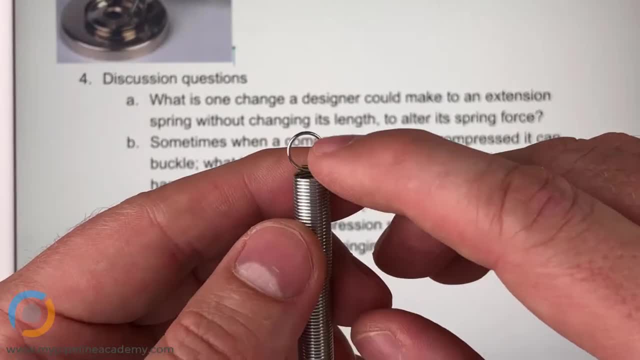 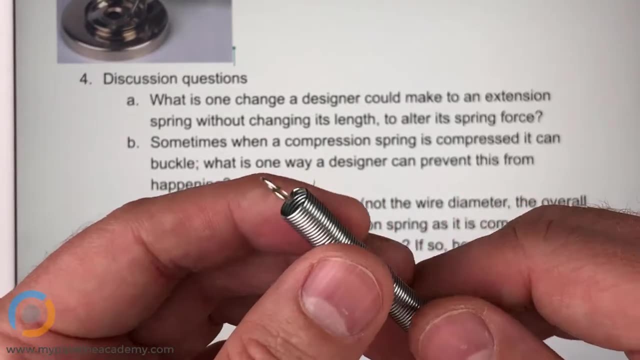 Maybe instead of a 30 thou thick or a 30 thou wire diameter, we could use a 20 thou wire diameter or a 40 thou wire diameter. If we were to use a 20 thousandths of an inch wire diameter here, what do you think would happen? 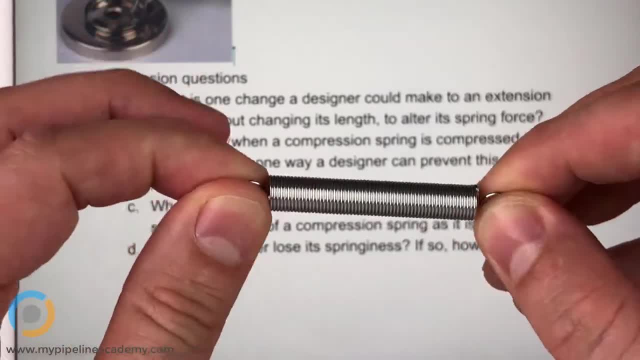 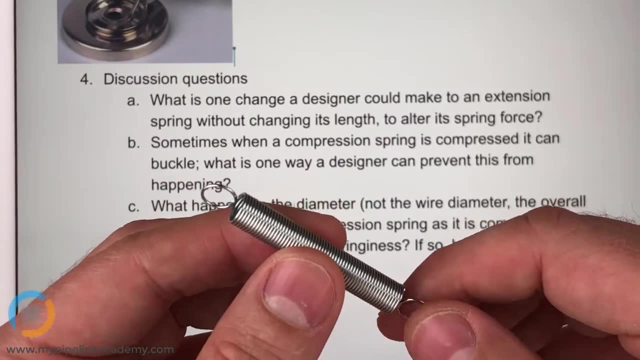 Would the spring constant? would the force be higher or lower? So you're saying, if the wire that makes up the spring is thicker, what would happen? Yeah Well, it becomes a stronger spring. So in this case it's more resistant to being extended. 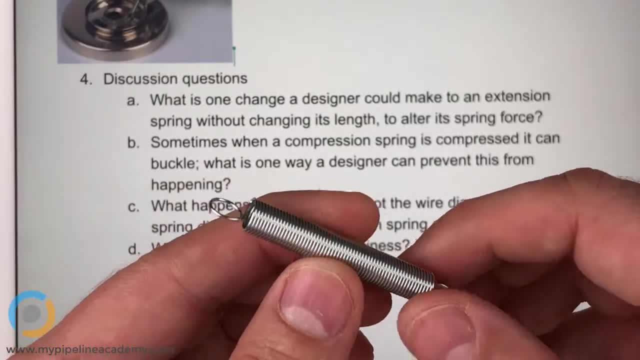 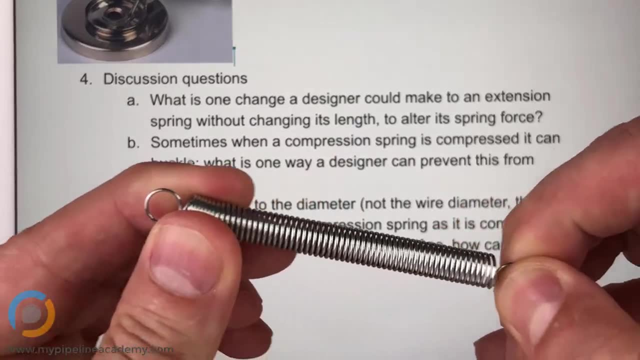 Yeah, with a thicker wire. Yeah, If you were to use a thinner, like a smaller diameter wire, then it would have less resistance, less force And, as a designer, more often than not you're going to be working with off-the-shelf springs that already exist. 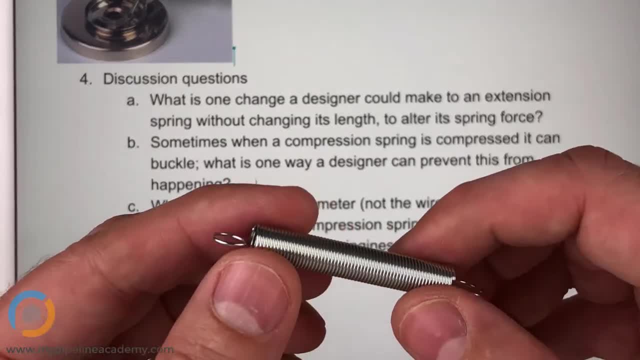 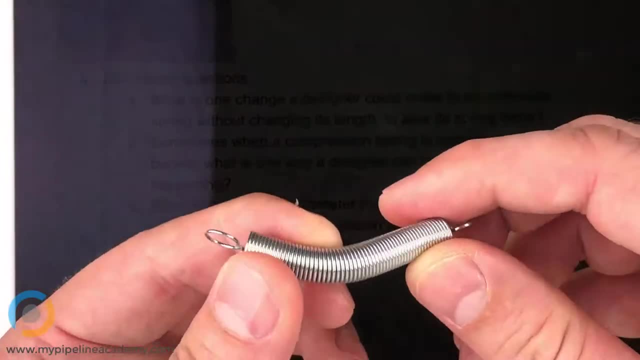 But occasionally you'll have to design your own, And so sometimes you might have the freedom to specify what diameter the spring is, And even with off-the-shelf springs there are so many of them you would never be able to memorize all of them. 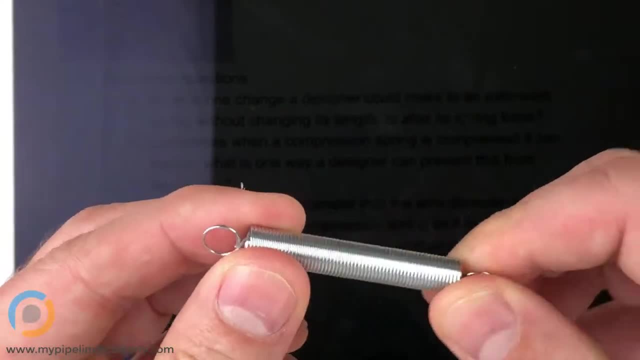 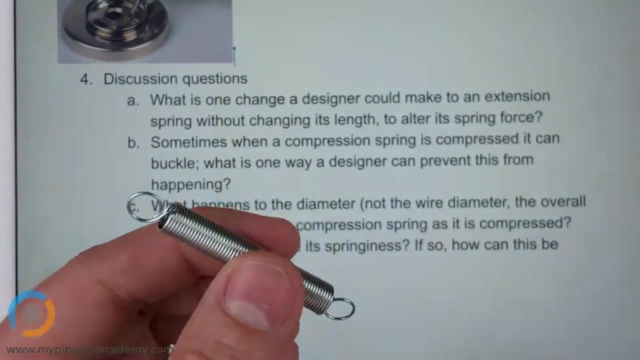 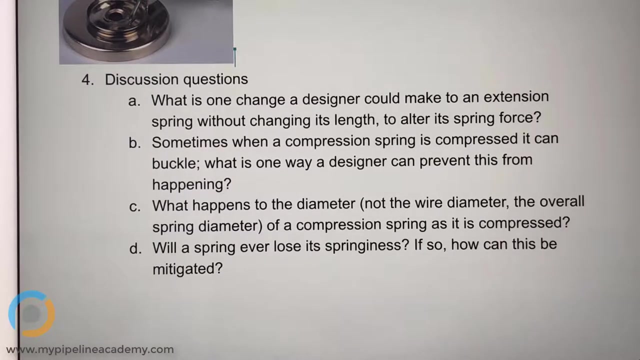 There are thousands of them. There are different lengths and materials and wire diameters and coil diameters, And so you just go to a website and look up what's available and find, hopefully, something that works- Perfect, Okay, So let's see the next one here. 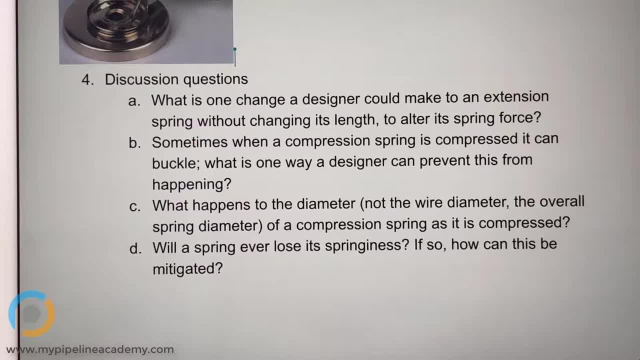 Sometimes, when a compression spring is compressed, it can buckle. What is one way a designer could prevent this from happening? First of all, the term buckle- Is that clear? No, So the buckling is Right, It's compressing. 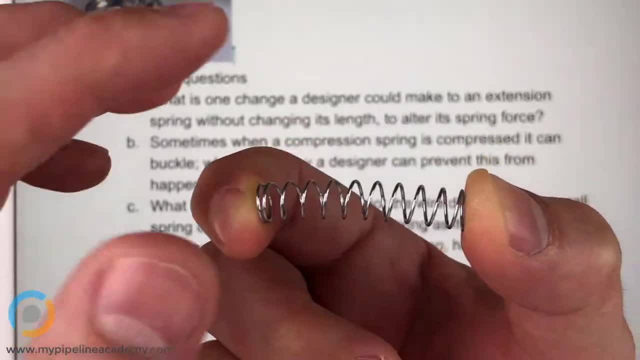 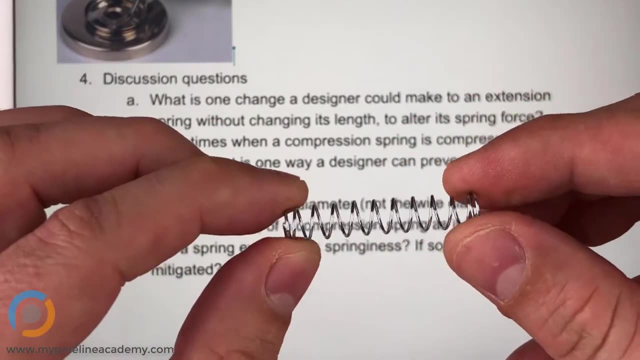 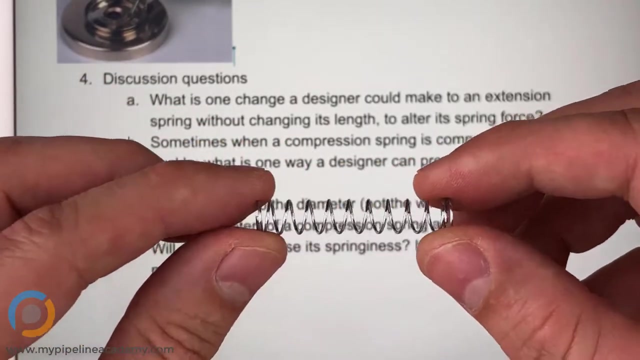 It's compressing And then, Oh, Buckled, That's buckling. And that happens not just with springs. It can happen with anything- beams of wood or metal, poles, rods- But we're talking about springs today. So what is one thing we could do in some kind of design application? 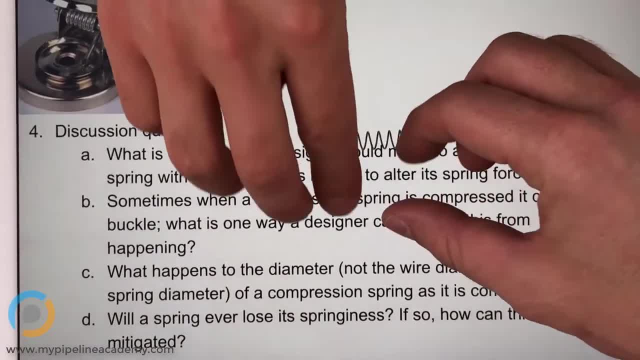 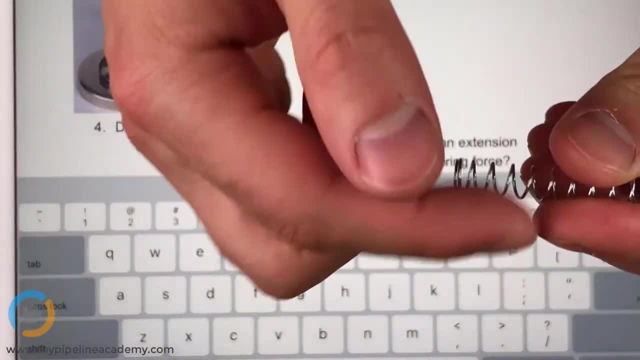 to prevent a spring from buckling, I'd say, maybe have something that goes in through the middle of the spring that holds it in place, or something on the outside that holds the spring in place. Bingo, Yep, That's exactly right. 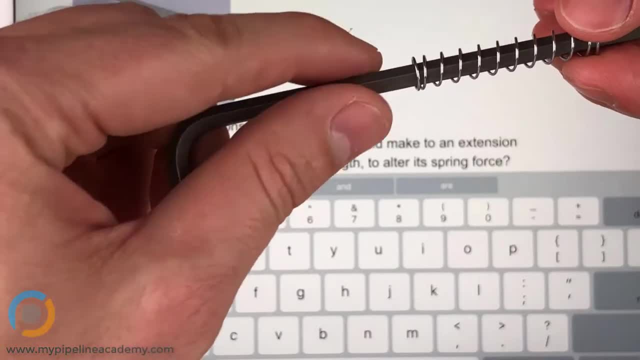 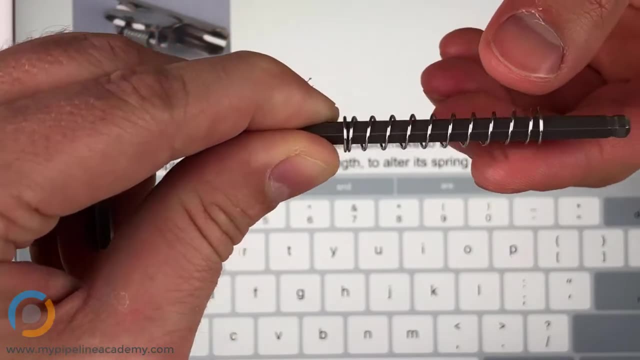 So if you had something like that that goes on the inside, why don't you compress that spring? now push it towards my finger. Yep, It doesn't buckle. Yep, It's held in place. Nice, And that's a really common method of preventing a spring from buckling. 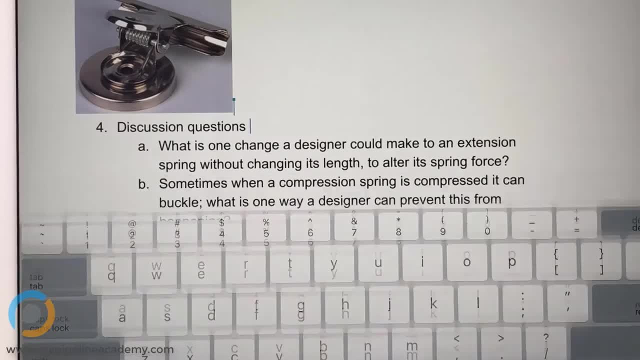 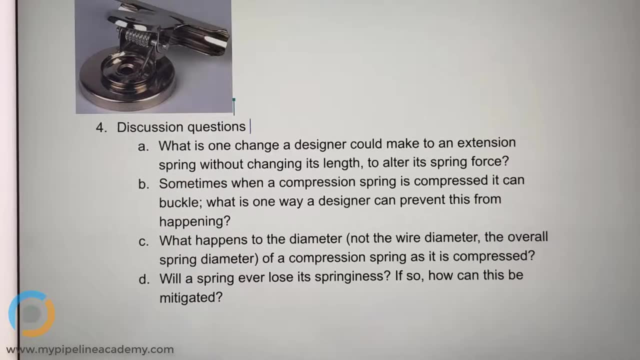 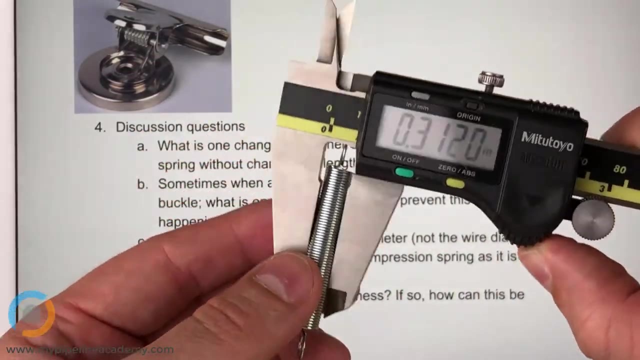 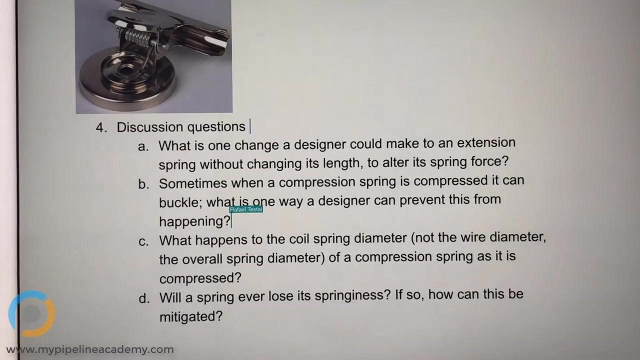 Okay, next, What happens to the coil diameter, Not to the wire diameter, but to the overall spring diameter? So this measurement right there. What happens to that diameter when- And let's actually talk about a compression spring, When we have a compression spring here? 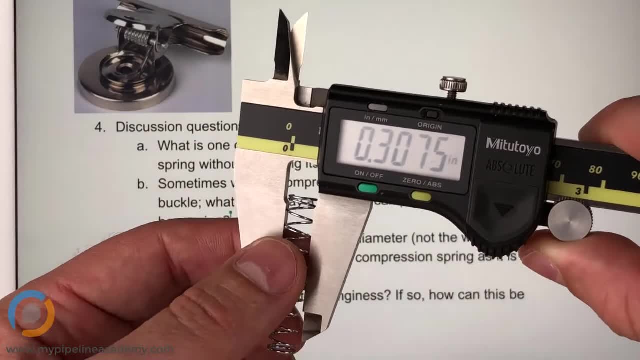 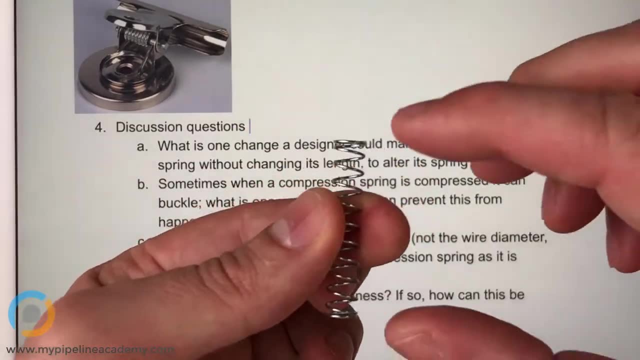 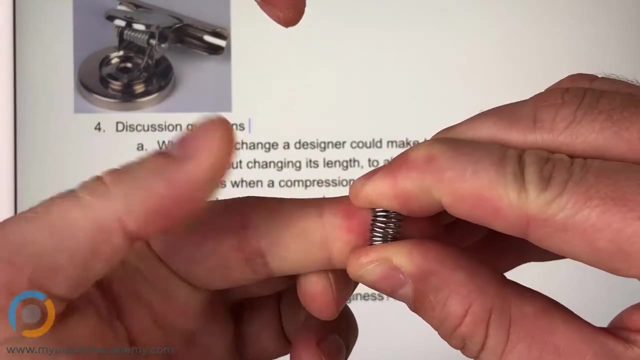 we've got some coil diameter- Okay, 0.3075 looks like. What happens to that diameter? Does it increase or decrease? when you compress that spring Like that, It gets a little bit wider. I suppose It does, You're right. 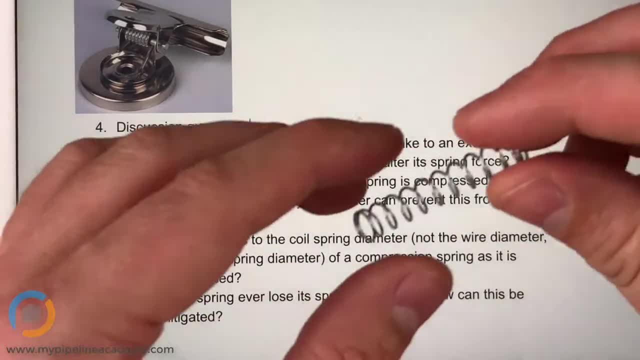 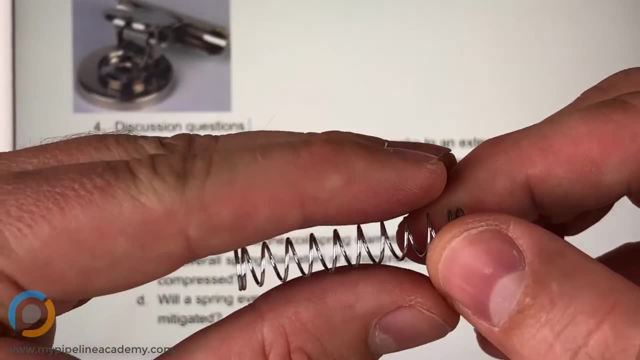 Yep, it gets a little bit wider, And so that's something that you need to keep in mind, because sometimes you might design something with a pocket, you know, that holds the spring on the outside, like that, And you just need to make sure that it's not so tight. 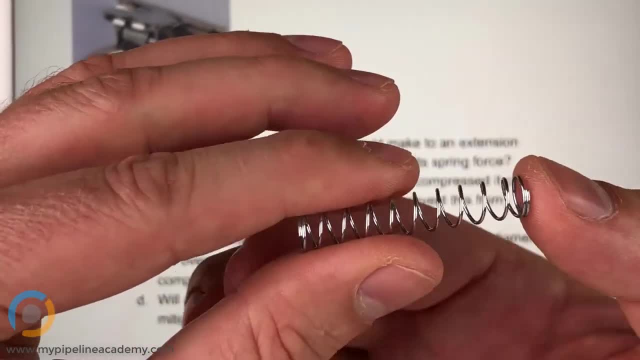 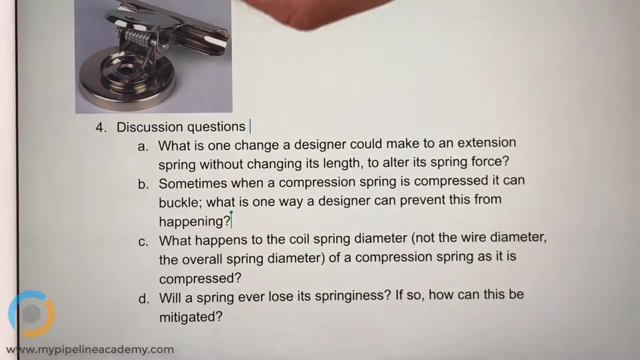 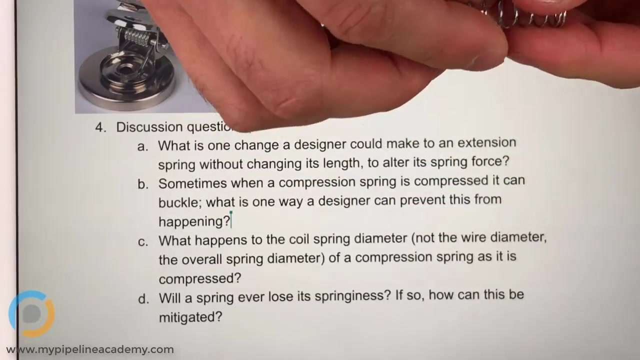 that that spring diameter doesn't bind, the coil diameter doesn't bind against the hole in your part when it gets compressed? And does that measurement as to how wide the diameter of the coil gets shown on MagMaster? I can't remember off the top of my head right now. 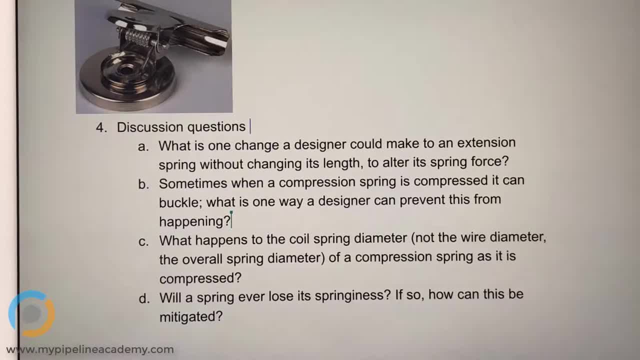 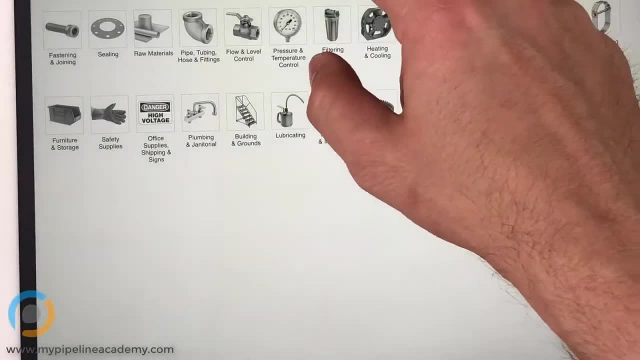 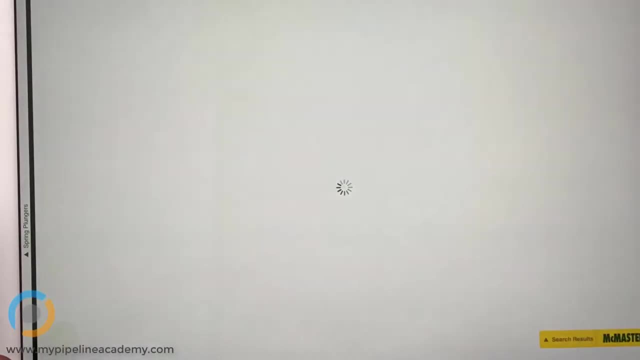 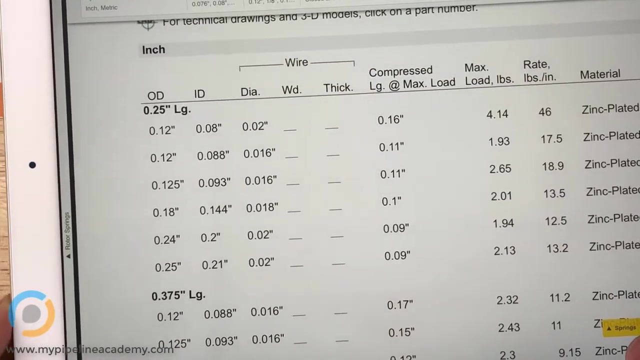 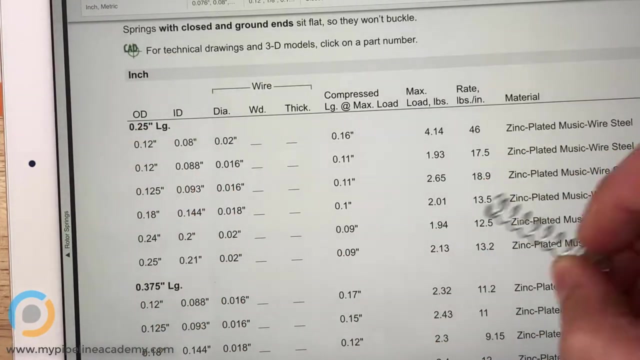 I want to say no, Should we check? Let's check it out, Let's check, Okay, So here are some specs for compression spring. We've got the OD, We've got outer diameter, which is that coil diameter, The ID, which is inside the coil diameter. We've got the wire diameter itself, Compressed length at max load. max load: Here's the spring rate, pounds per inch. I don't see Sometimes they'll tell you what is the minimum hole diameter in which the spring can fit. 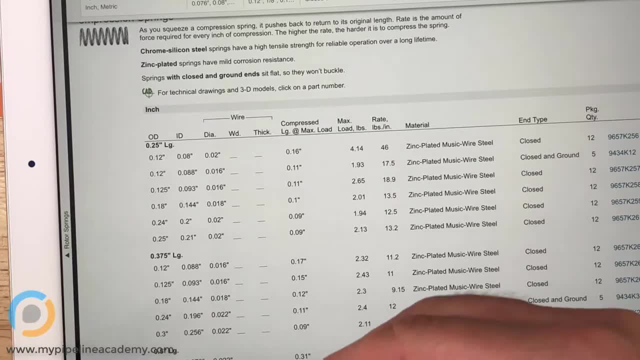 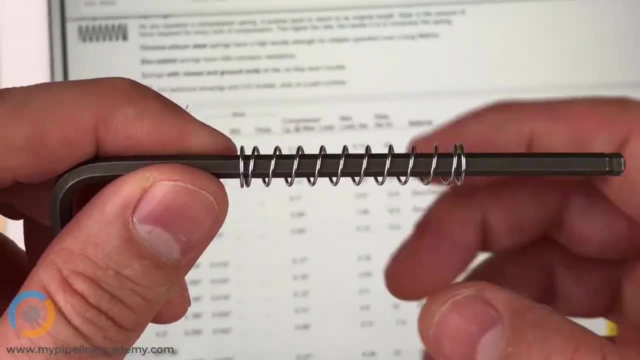 or what's the maximum mandrel diameter. That is, whatever you have on the inside of it. They might tell you what's the maximum mandrel diameter you can put. So it looks like I don't see it here on the MagMaster mobile app. 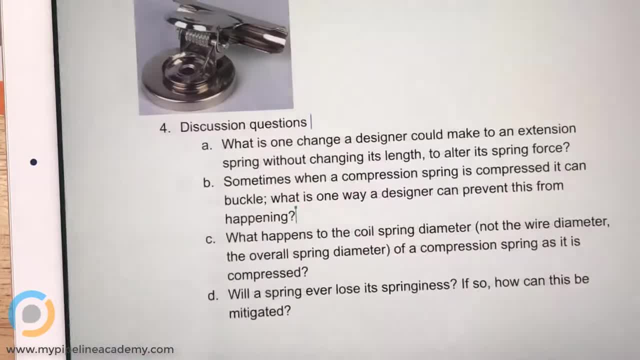 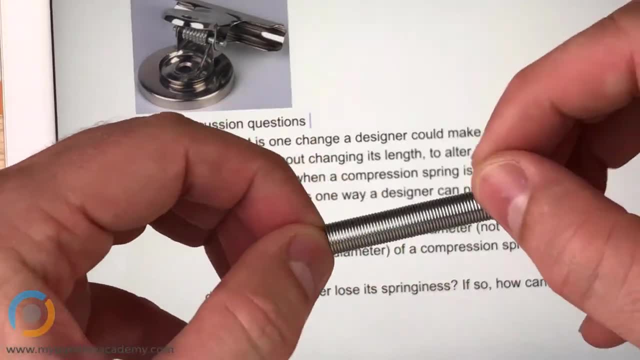 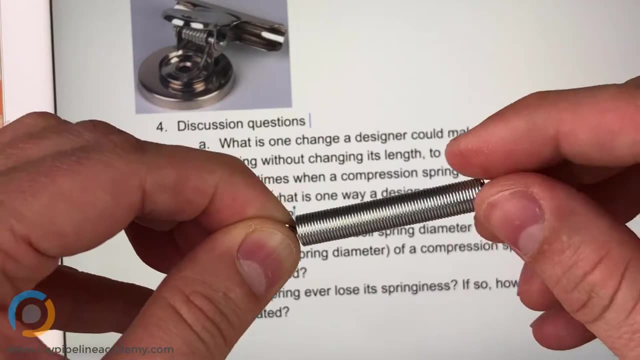 Okay, And the next question? Okay, Will a spring ever lose its springiness? Right, If I pull on this extension spring and let go, it snaps back. That's what a spring does. So if I do this 100 times, is that springiness going to go away? 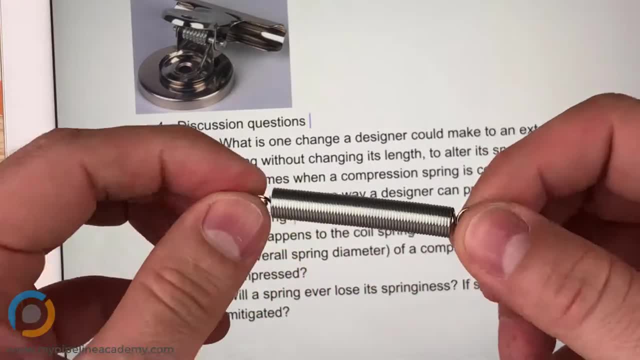 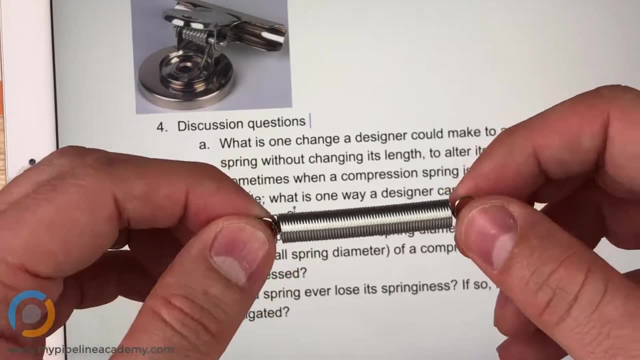 What do you think? I think so. It's not an everlasting material, But I think what one can do is to prevent it from the weather. maybe weather conditions, water, maybe put a coating on it, if it's possible, I don't know, guys.